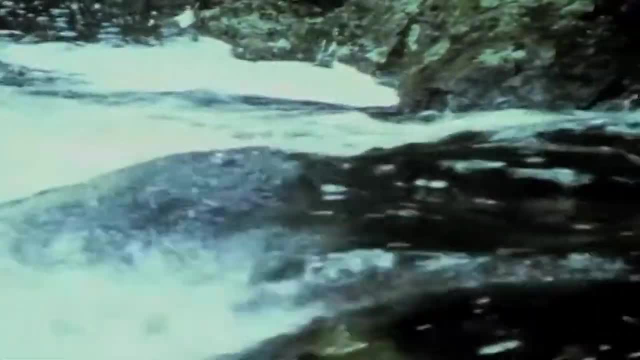 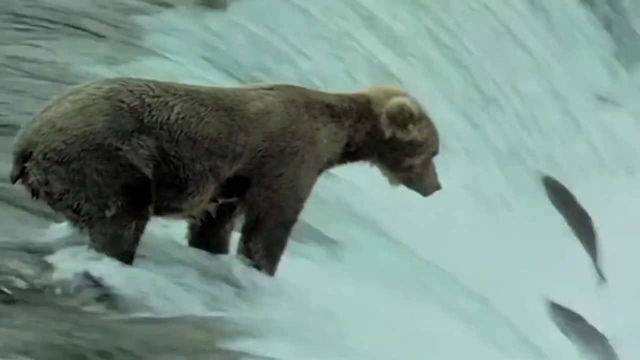 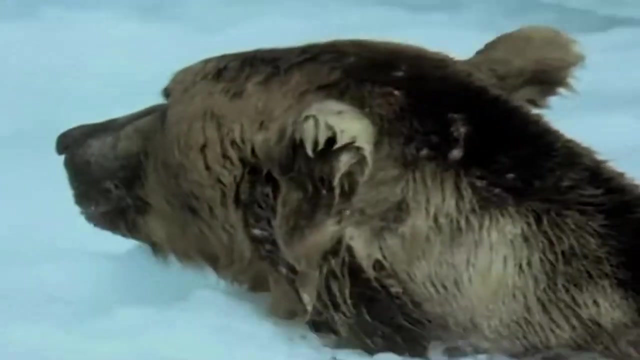 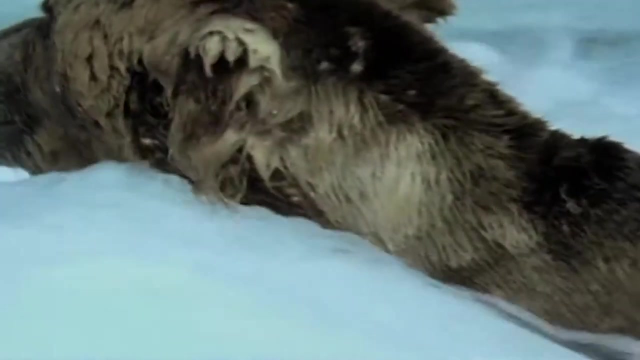 They struggle up the waterfall just to encounter a more dangerous adversary: The grizzly bear. These grizzly bears assemble at the rivers, eagerly awaiting the salmon's expected return. And the salmon do not disappoint. For the skilled grizzly, they're an easy meal. 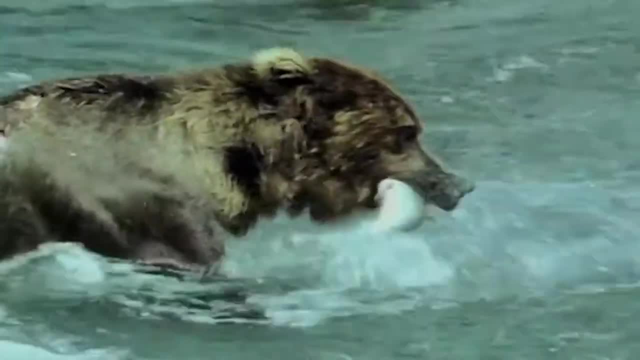 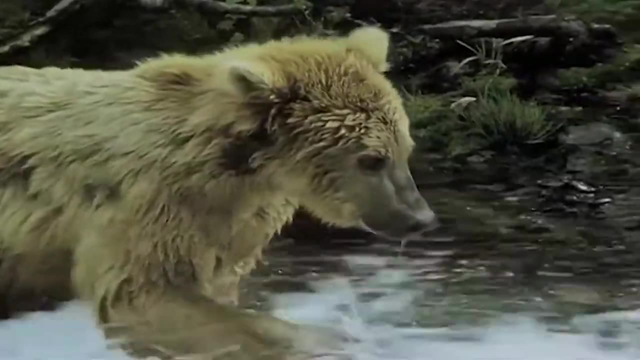 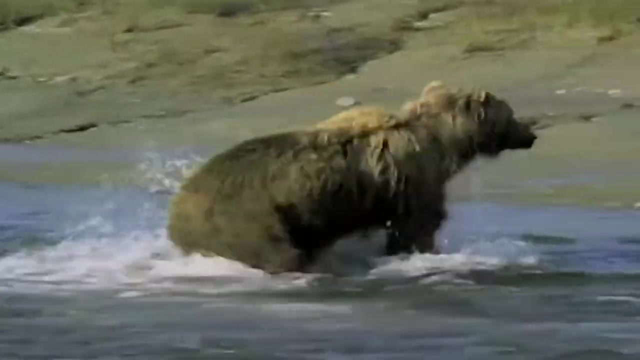 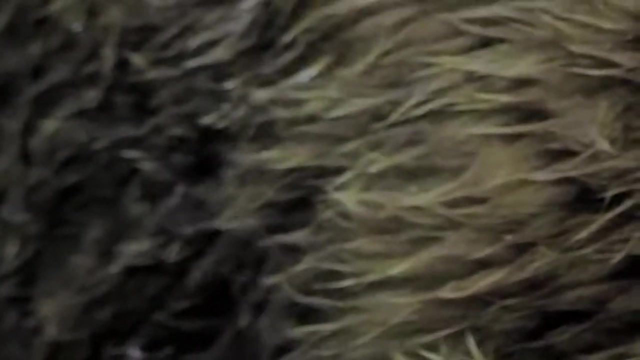 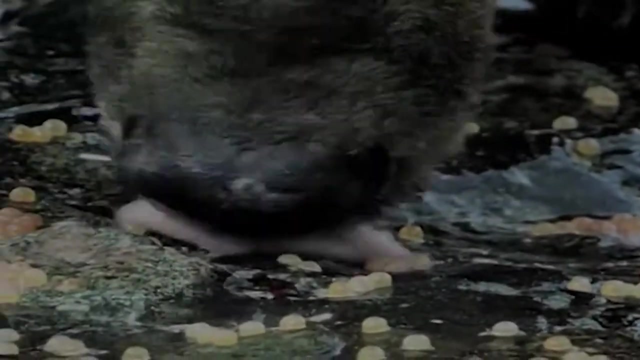 The younger bears, though, have a tough time catching the slippery fish. Unfortunately, many salmon lose their lives at this stage. It is caviar for the bears, but the death of these eggs marks an abrupt end to the future of the salmon. 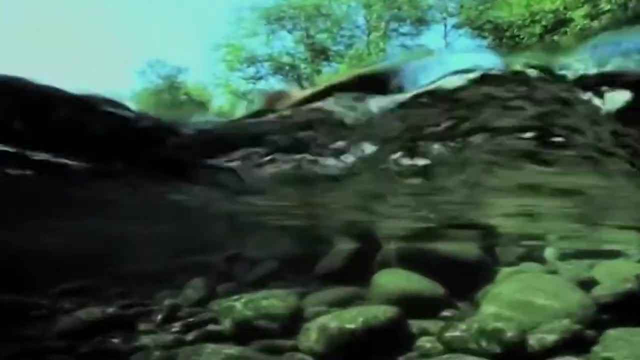 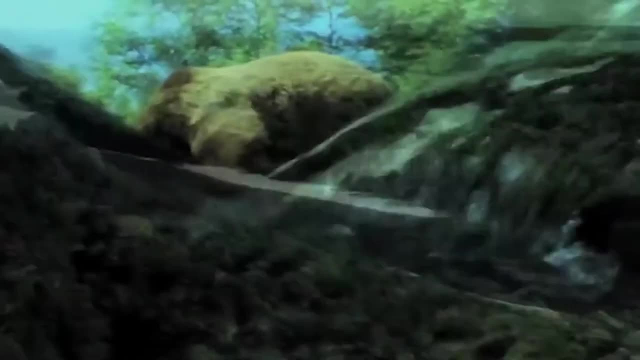 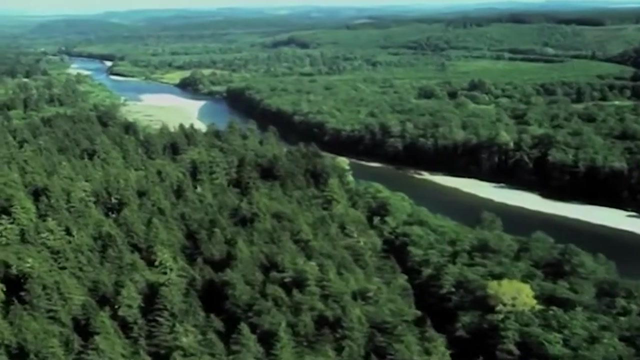 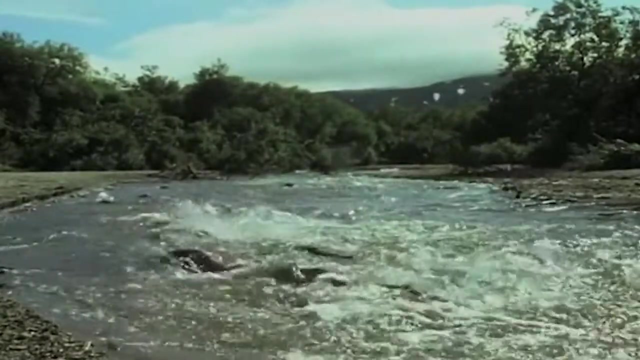 Several of these bears have died. Several of them are successful in escaping these predators and continue with their thousand-mile journey. As the rivers converge and the waters become shallow, their sharp sense of smell guides them to the breeding grounds where they were born. The urge to procreate motivates these fish to overcome the relentless force of the current. 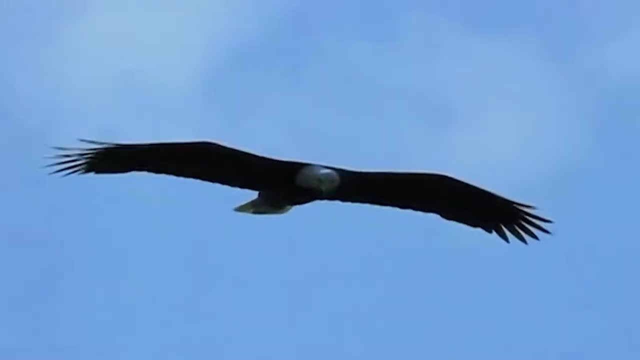 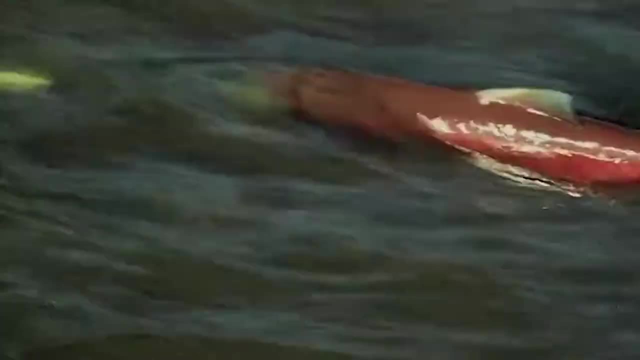 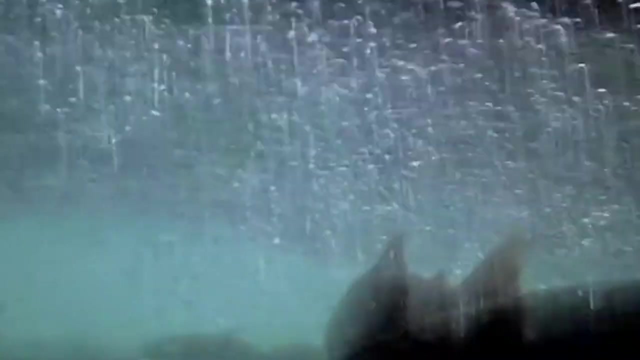 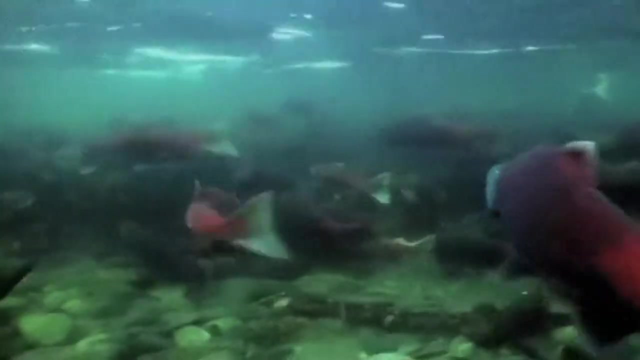 as they continue on their extraordinary mission, The salmon also become easy targets to aerial predators. due to the shallow waters Just prior to spawning, the sockeye salmon undergo striking changes in their colour and shape. The males' jaws transform and grow a vicious set of teeth. 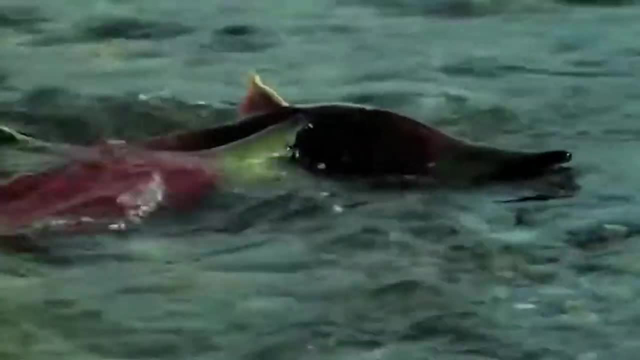 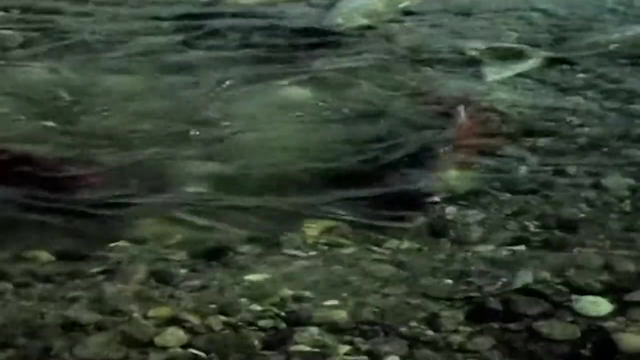 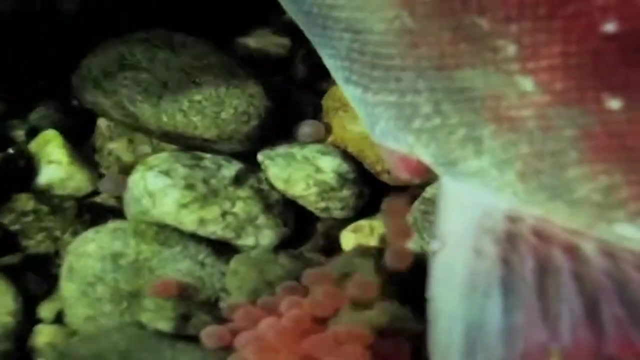 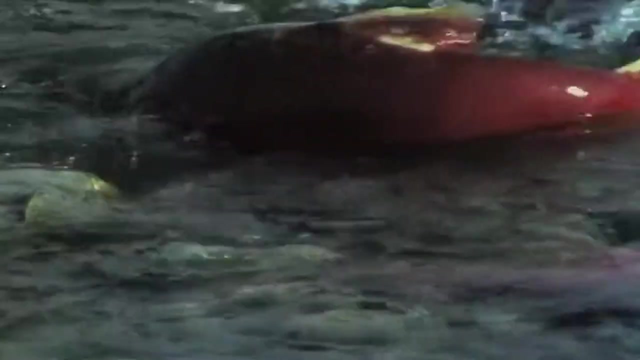 They have to compete with each other to win the right to the best females. Once paired, the female digs a shallow nest on the riverbed before laying her eggs. The male then fertilises them, Having mated. finally, thousands of heavily fatigued salmon now perish in these waters. 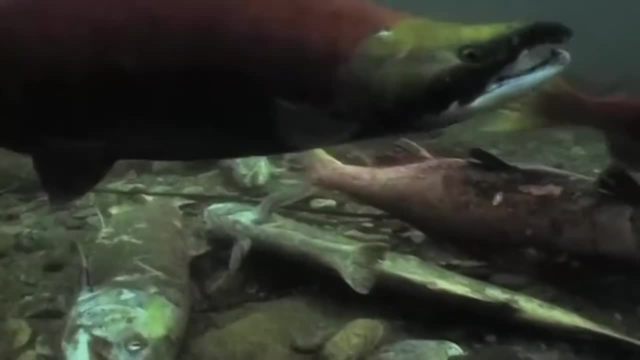 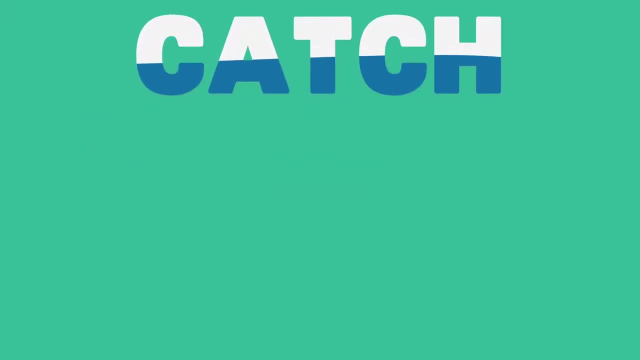 The adventure is over. The sockeye salmon die in the very same riverbeds that they were born in. Subtitles by the Amaraorg community.